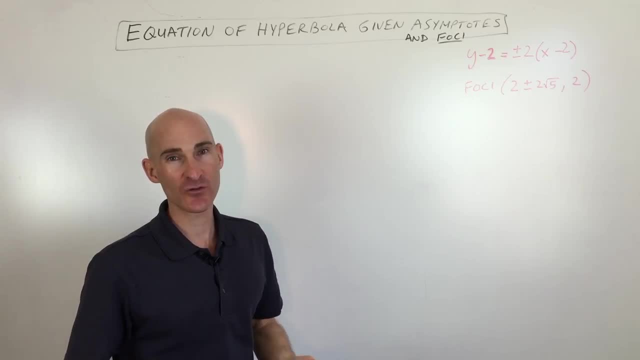 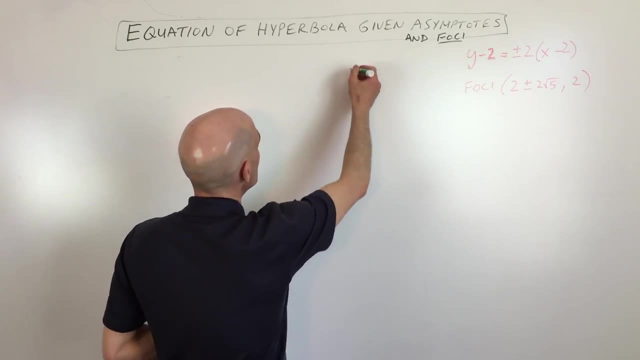 And what I recommend with all these types of problems is just to draw a sketch. So if you draw a sketch, sometimes it'll help you to figure out the other pieces of the puzzle. So let's go ahead and do that. So first thing we have is: okay, we've got a coordinate axis and we know. 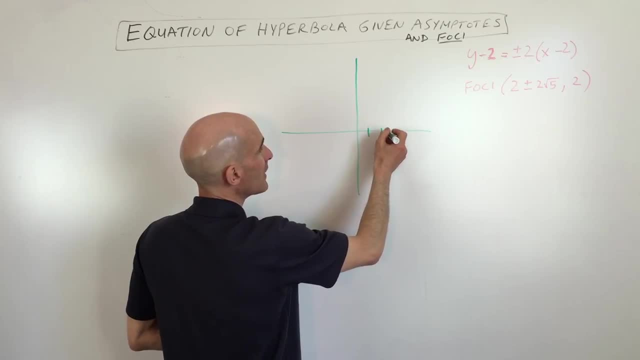 our foci are at 2, okay, plus or minus 2 root 5, comma 2.. So we know we're going to be going up 2 here. okay, that's the y value, but then we're going to be going 2 root 5 to the right okay. 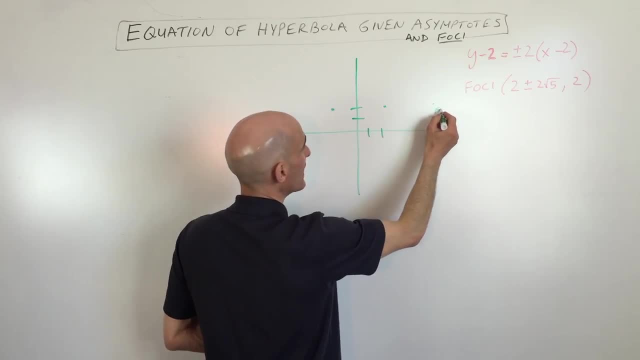 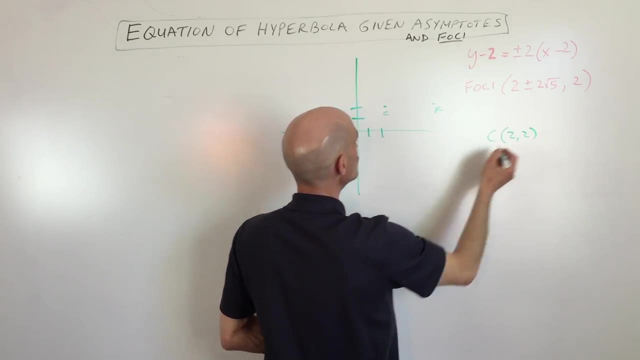 and we're going to be going 2 root 5 to the left. Those are the foci, okay, and this is the center. Okay, so you can see the center is going to be at 2 comma 2, okay, because it's halfway in between. 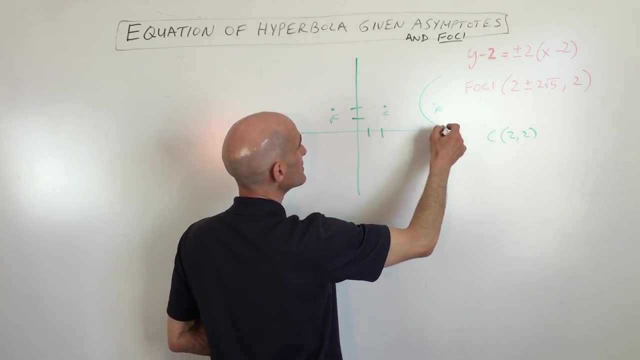 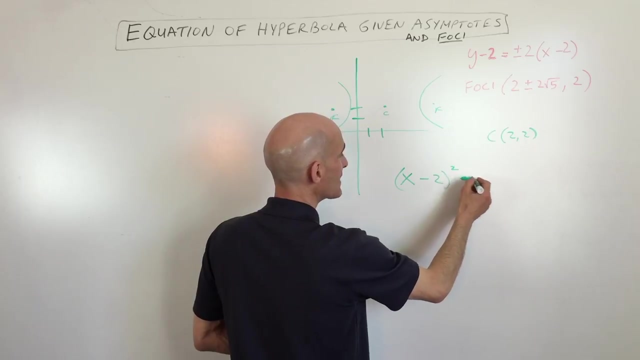 the foci, and we know that our hyperbola is going to look something like this and like this, approximately. okay, So now let's put together what we know so far. So we know that x minus 2 squared, plus minus for hyperbolas, plus for ellipses, y minus 2 squared. 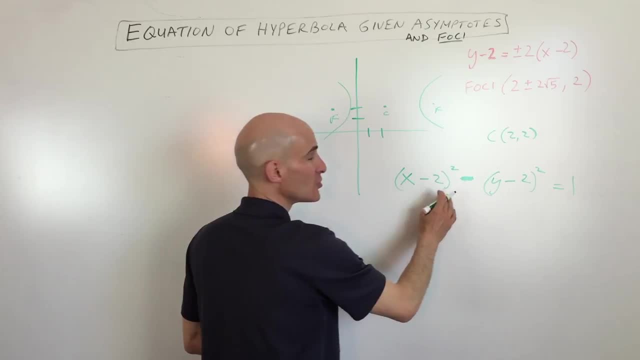 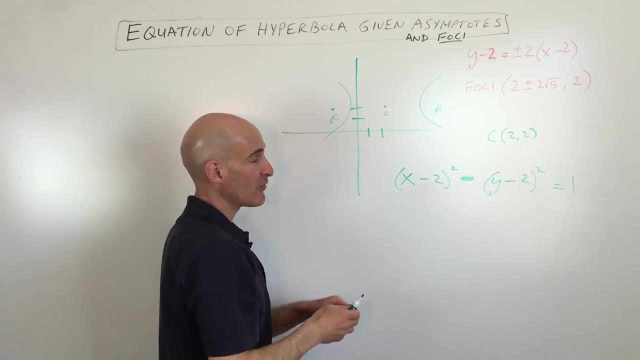 equals 1, okay, So we've got our center: 2, 2.. The x squared term is the positive term that comes first when it's opening left and right. If the hyperbola is opening up and down, then the y 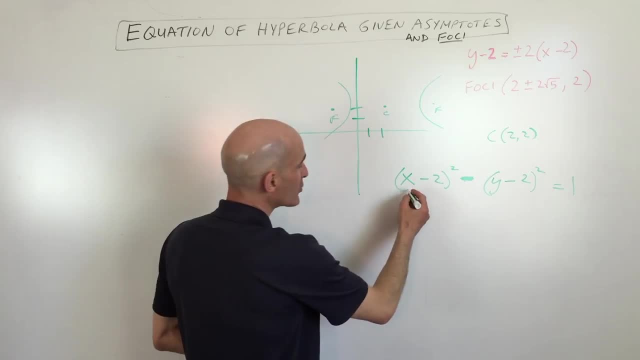 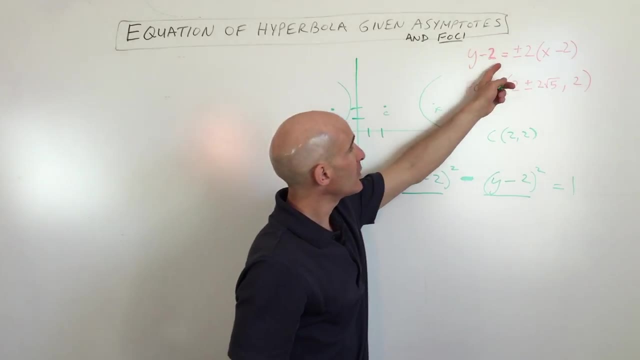 squared term would come first. okay, So are you with me so far? And then what we're trying to do now is we're trying to find the denominator. Okay, the a squared and the b squared- Okay. now we look at our asymptotes here and we can notice. 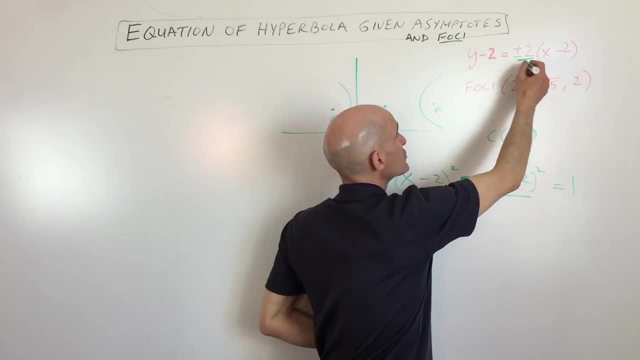 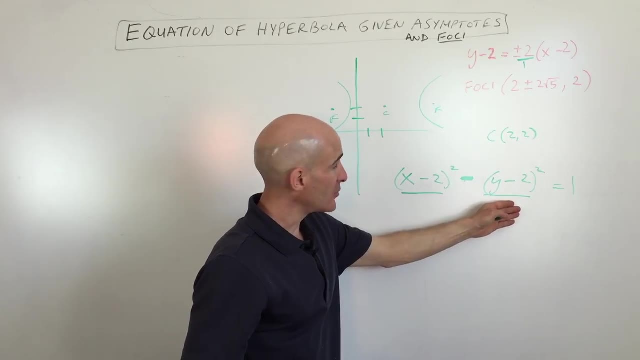 that the slope is 2, and plus or minus 2 over 1.. Anything divided by 1 is itself, and we know that the ratio of the quantity that's underneath the y term divided by the x term is going to be the slope of the asymptote. So this is going to be the rise and this is going to be the run. Now, 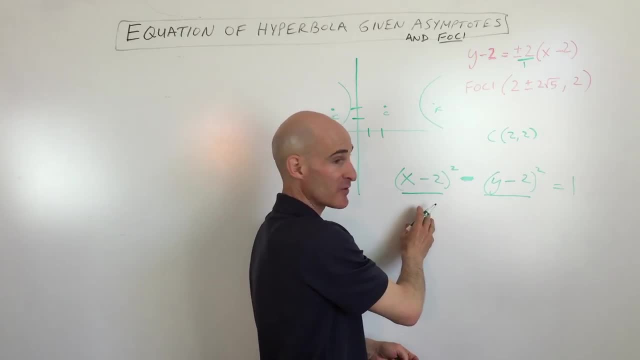 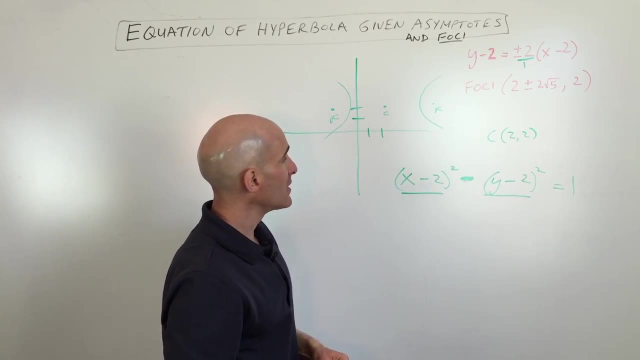 if these terms were reversed, then we want to take the determinant here, okay, the one that's underneath the y value divided by the one underneath the x value. So what we're going to do here is we're going to say, all right, this is a squared, this.